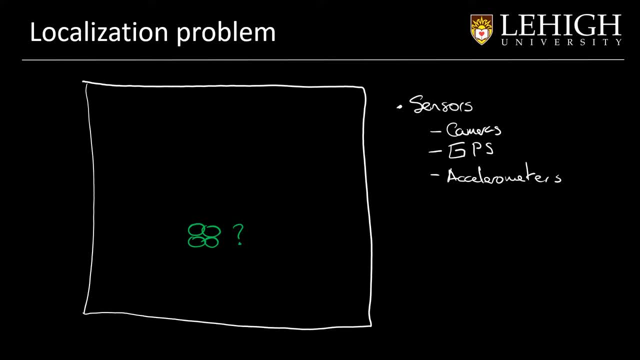 even compass. there are many internal sensors that the robot can use. In this context, the main question is like: how can we use these sensors to identify the location? Even the GPS is inaccurate. right, The GPS can give an error of around three meters. 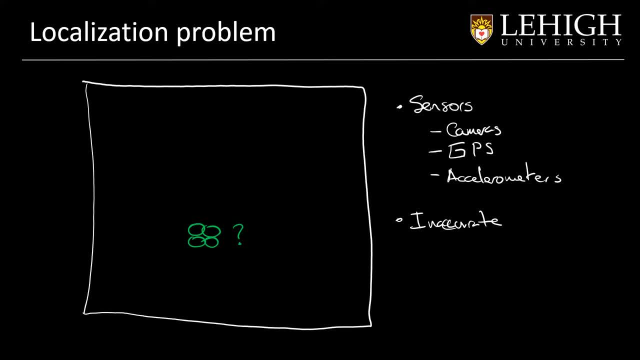 If we talk about a self-driving car, three meters will be the difference between being inside the road or outside the road. So that's the main question And in this context, we are going to assume that we have some landmarks. Let's see that we have some trees in the environment, just to help the robot to identify where it is. 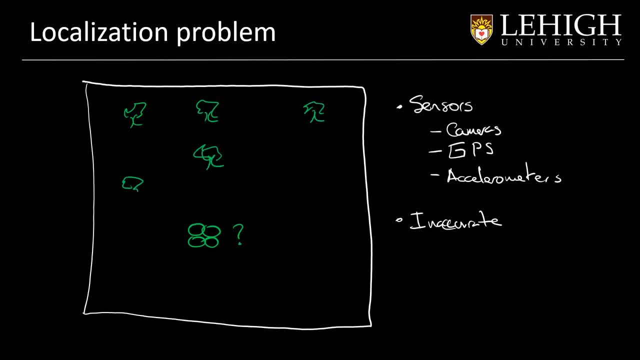 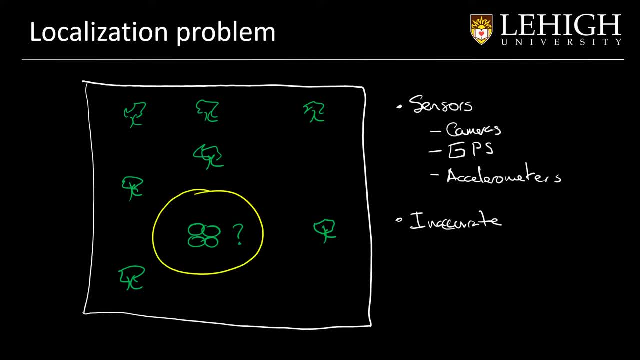 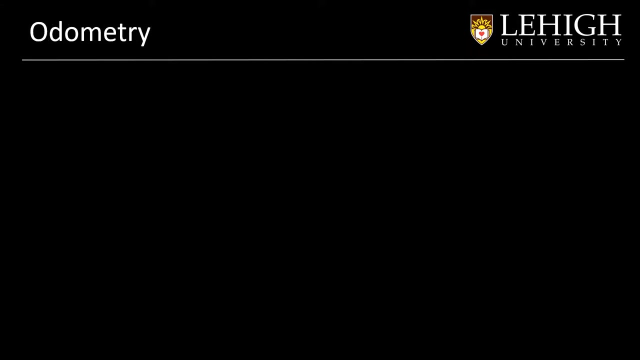 So let's take a look at the map. In the case, for example, of the camera, the camera has a range, So that's what we call the sensor footprint, And this is our drone. The first part that we will use here is about 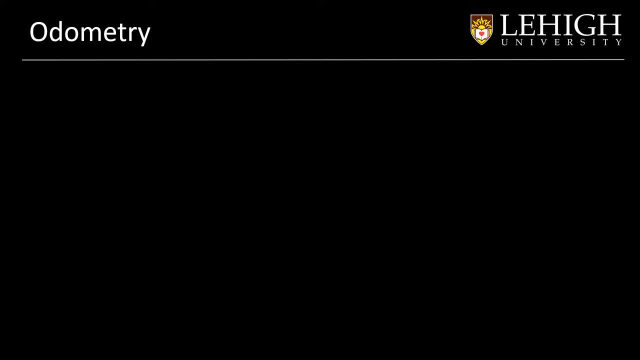 predicting the location or how to use odometry in order to estimate where the robot is. Let me give you another example that is pretty simple. Let's assume that we have a planet, environment here And let's do a simple exercise. There is a human and the human has the eyes covered. 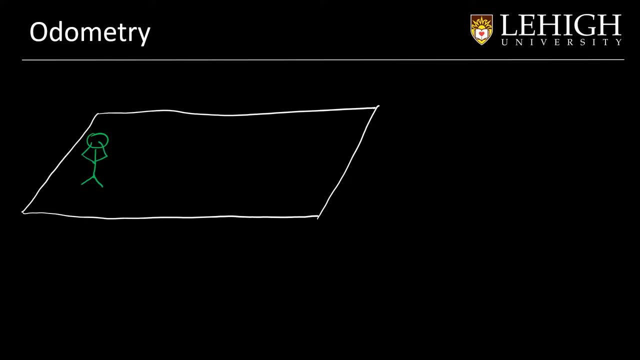 You can imagine that you are that human. And now what happens if the human gives three steps? You can guess. you kind of can guess where you are going to be: Maybe here, but maybe here, or maybe here, maybe here, maybe here, right? 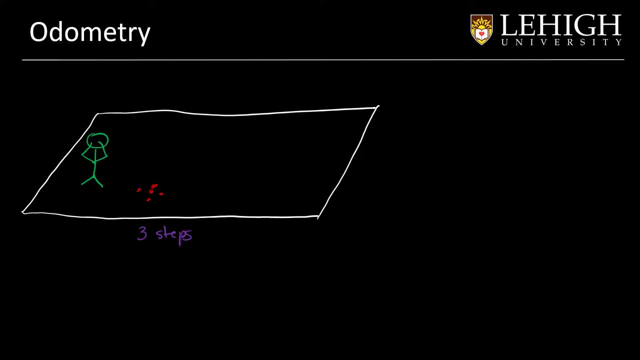 That happens because the length of our steps are not perfectly synchronized or aligned Like we don't have an accurate measure of the length of the step, So there is an error involved there. If we have more steps, let's say that we walk for 10 steps. 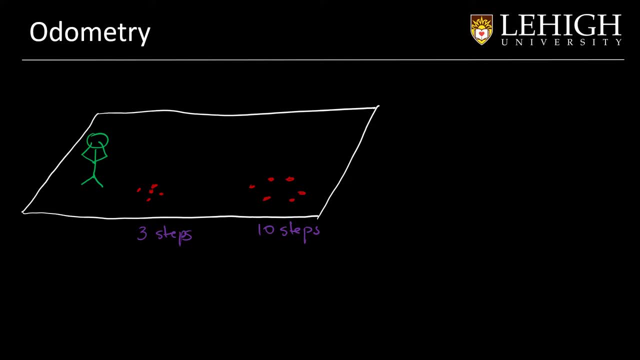 then the error will be higher. right, We can hit here, hit here. These are all the places. This is where we can be And we can assume, or we can try to start to model that type of error, Like our error will be inside this ellipse and if it goes farther, it will be inside this ellipse. 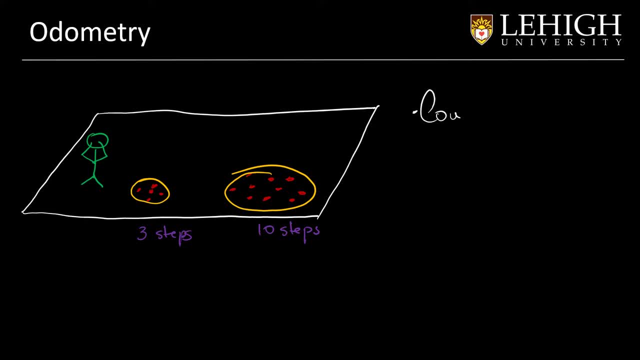 So this is just basically counting steps. So in robots, we can use something similar using odometry. Using odometry, we can use something like the If this is the state of the robot with the x and y coordinates. 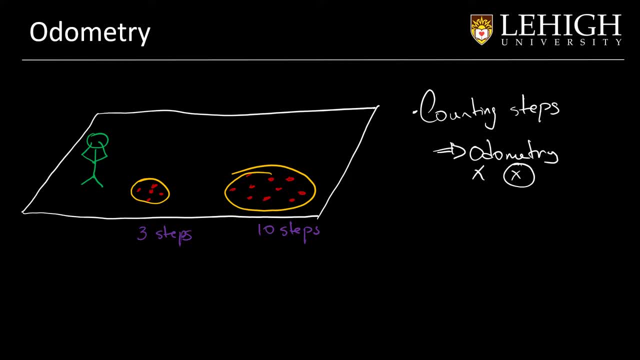 and we know the speed of the robot, we can integrate the speed to obtain the new location of the robot. So the So the. The goal of using this prediction is basically estimating a new location based on the control input. So let's say that we want to know the speed. 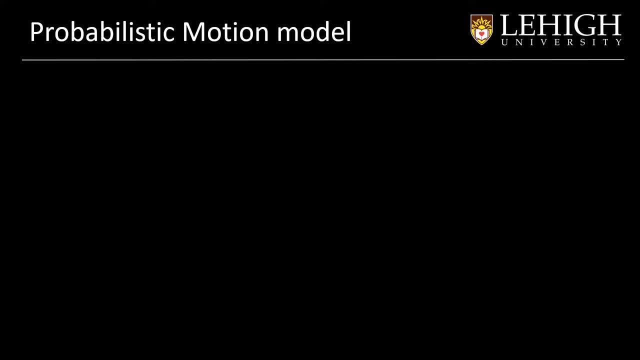 So we can use a little bit of computation to calculate the speed of the robot. In mobile robots we have something similar as counting steps that is based on odometry. So in mobile robots we have something similar as counting steps that is based on odometry. 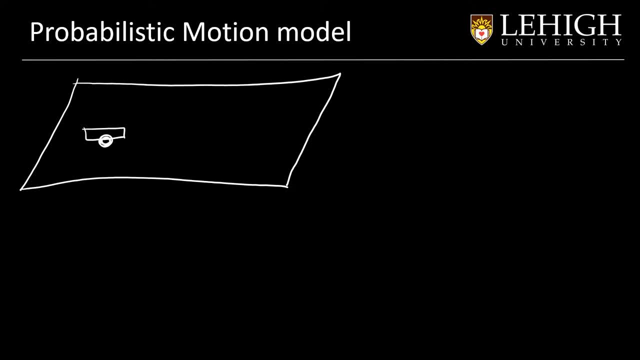 For example, if we have a differential wheel drive robot, For example, if we have a differential wheel drive robot, this robot will move forward If the control input is moved forward, If the control input is moved forward, If the robot is moving in this direction. 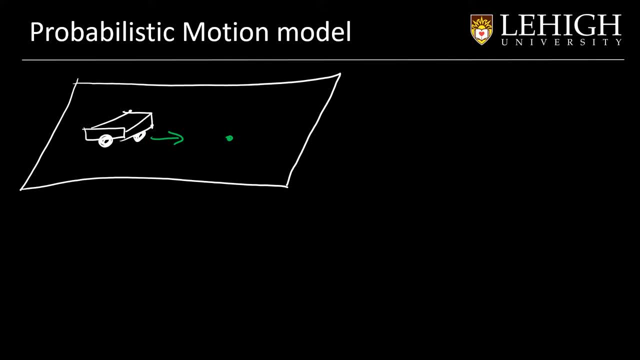 robot is perfect. it will fall here. if the wheels spin a little bit slower, they will kind of fall around here. but if one of the wheels is faster than the other, it will kind of fall here or here. if the error is very big, it will be like this, right and same for the other side. this is called. 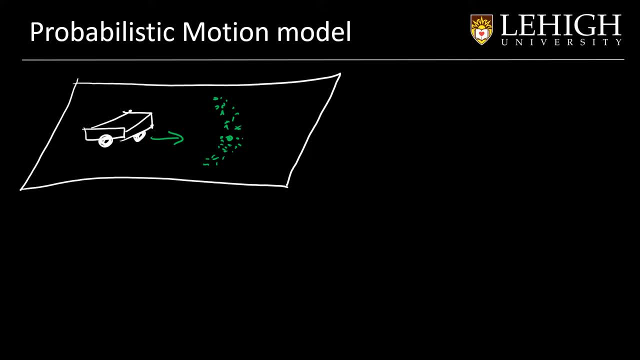 the banana shape error in a quadrotor and similar to the model that we will study today, will be something like this: we have the drone, it moves forward and we can assume that it will try to fall here, but sometimes it has some error falling from error breaking, and this will be kind of the distribution that we have. it will be a 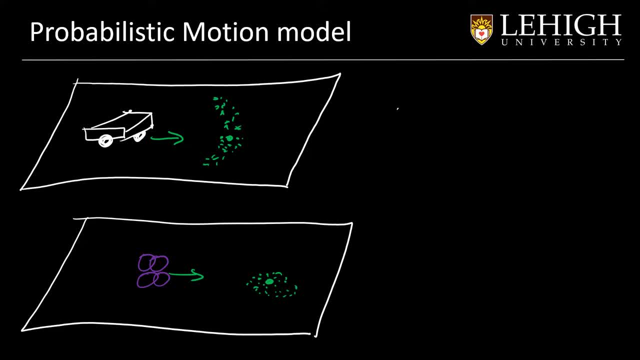 normal distribution. so in this case, what we have is: we want to know the probability distribution of x, given the previous time step, and the control input t. okay, so here we have that x is equal to x, y and x todos, our control input, based on this model, and if we assume that the model is linear, 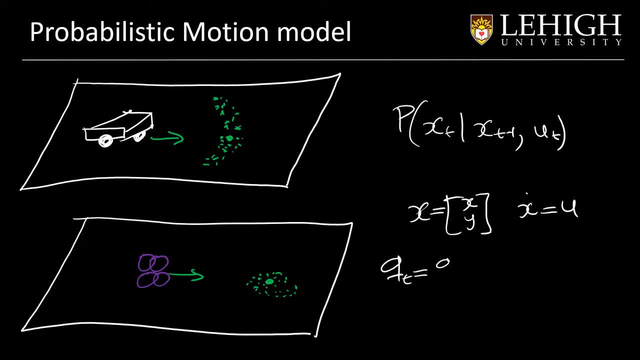 and very simple and simplified for holonomic robots. we will have this equation over here, where the new step is equals to the previous step, plus the integration of the pre, of the control input, which is the velocity during this time interval, plus the error, and we will assume that that error is just a normal function. 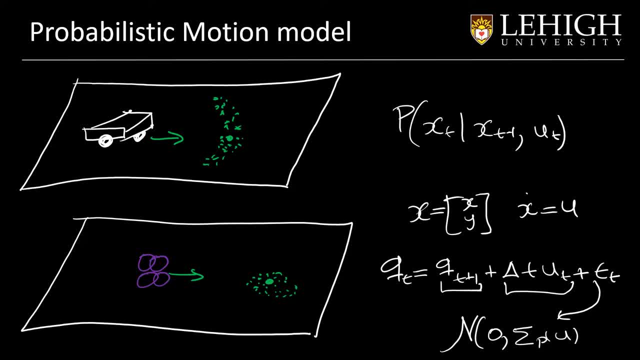 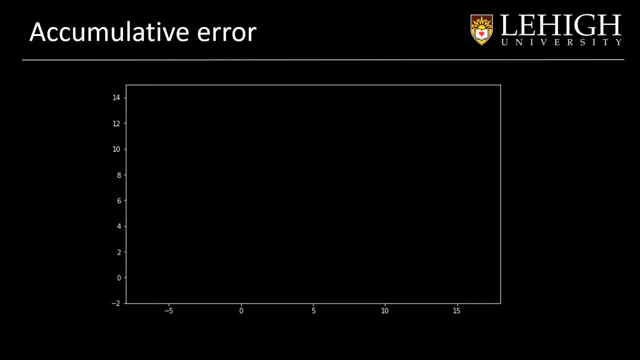 we will go in details later in this video. the main problem of the odometry is that the error will be accumulating while we move. for example, if we start in this location and we apply the following control inputs, what we are going to see in the end is that the error here, for example, for for the 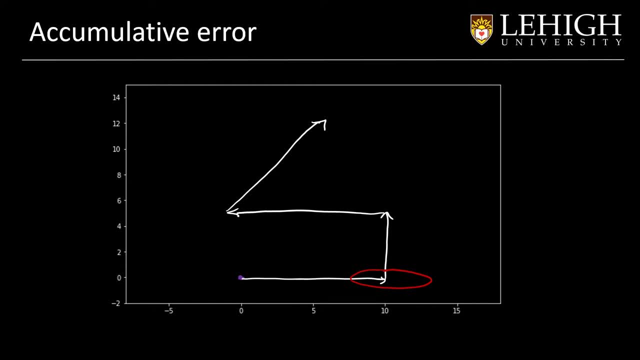 drone, the error is very small in the y axis, but when it breaks the error can be higher. so after the moosh, the, the movement, the robot can be here, or it can be here, or it can be here. it can be here right now. we have a range where the robot can be here here right now. we have a 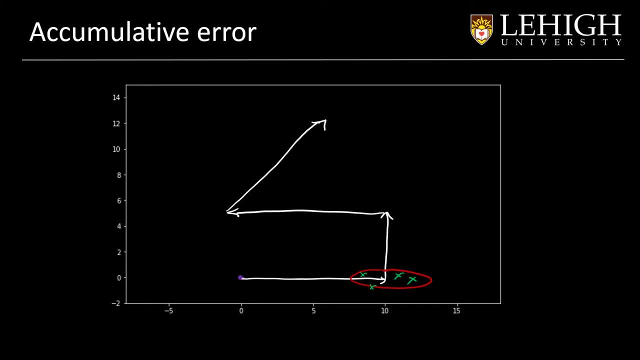 range where the robot can be can be. if we apply, if we move again, we will have an error around this ellipse, because if the robot was in this location, if it moves now, it will be here or maybe here, and if we combine all of them, we will have something like this: 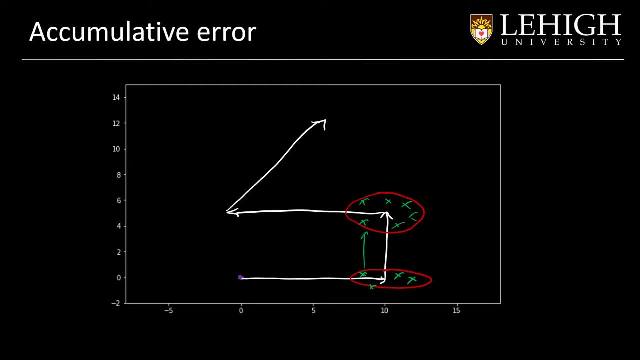 when we apply the next control input, we will go. our error will grow like this: and for the last control input, our error will be like this: very big, and if we continue, will continue growing and growing and accumulating. this is the clean representation of our ellipses and how it will be if we continue. 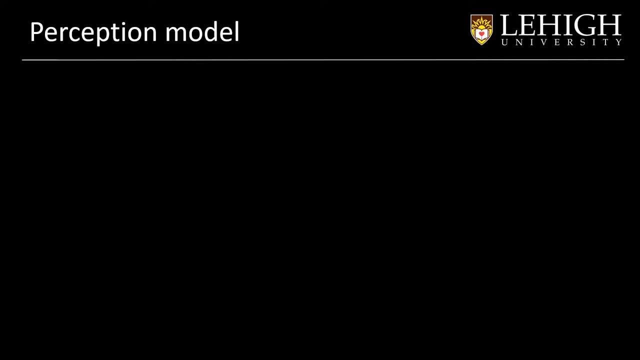 using the odometry. we know that the odometry is not enough if we want to have a good estimation of the localization, so we can use additional information, like we can use the map, and we can use additional sensors like cameras or GPS. and now let's come back to the 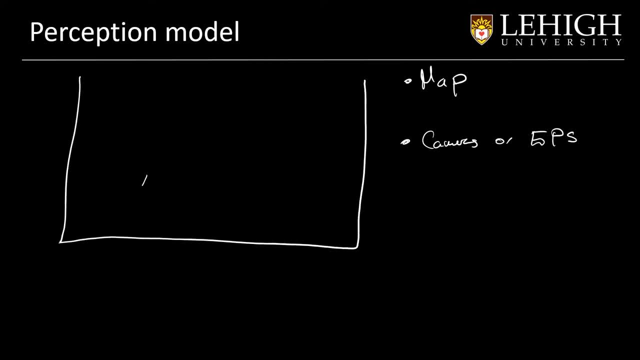 vehiclealet. so this, for example, is considering we can talk about our scenario where we have an environment and inside the environment we have some, some trees that are part of the map or they are landmarks. so if our aerial vehicle can see one of those landmarks, you will know, you will have a better estimation. 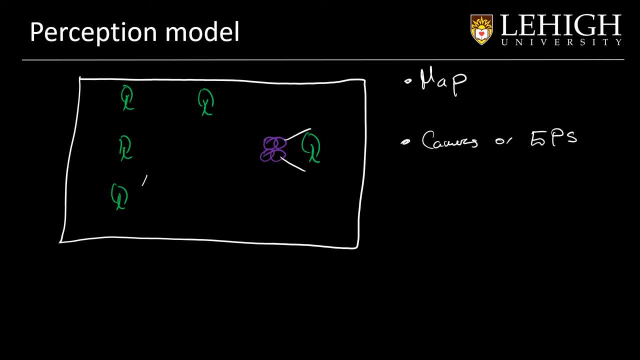 of where it is, the GPS, it will have an estimated estimation about what it is. so one way to model this in a very simple way and could be that the measurement that we get is equals to the real value of the robot, plus an error that we will denote as lambda t, and we can assume that that error is normal. 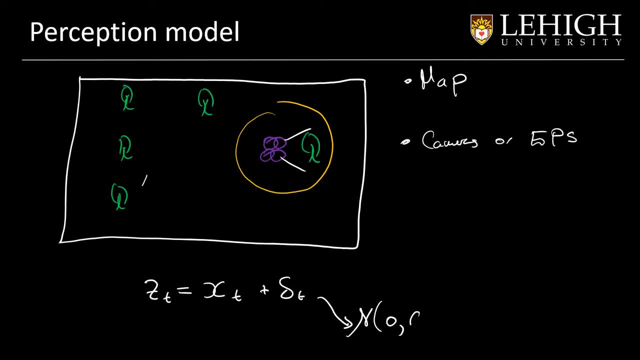 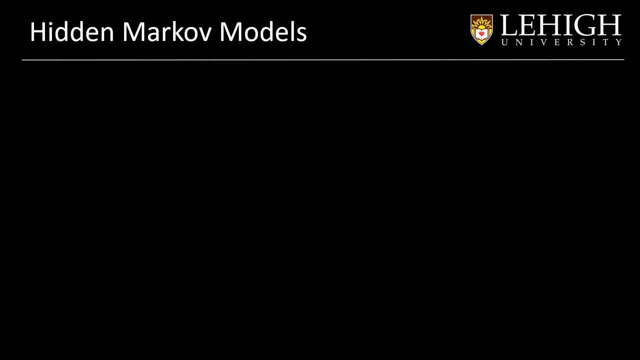 it's normal with meaning 0, and we will have a covariance matrix. okay, so this is basically to identify to. that's basically the perception model of the robot. now we will find a way to combine those two type of measurements that we can get from odometry and from the perception. 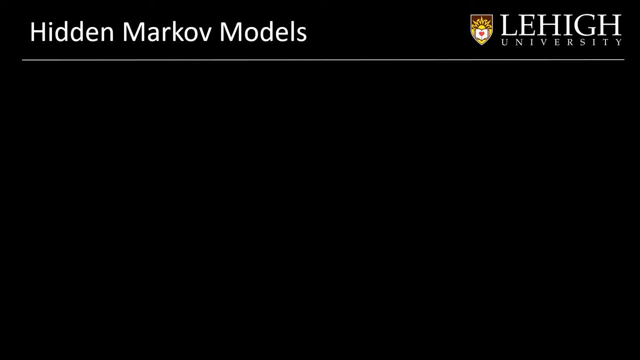 model. so what we have this is a hidden Markov model and this is the Markov models principally study base networks that change with time. so we have the state of the robot at time step 1 and it evolves to time step 2 and so on. it continues evolving with the number of time steps right the problem. 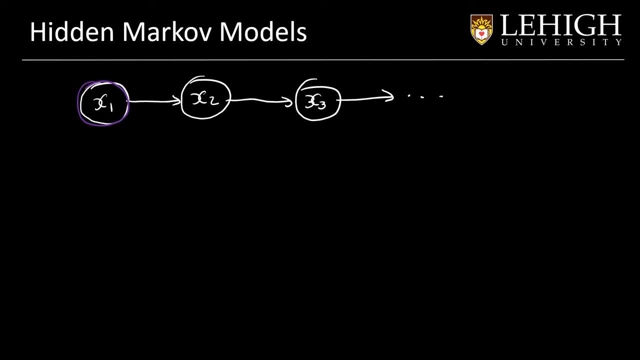 is like we don't know this, this is hidden. that's what is called the hidden Markov model, because we don't know that that state. this is just the base net representation of the mark hidden Markov model. it's a graph where the nodes are variables and they have a distribution. 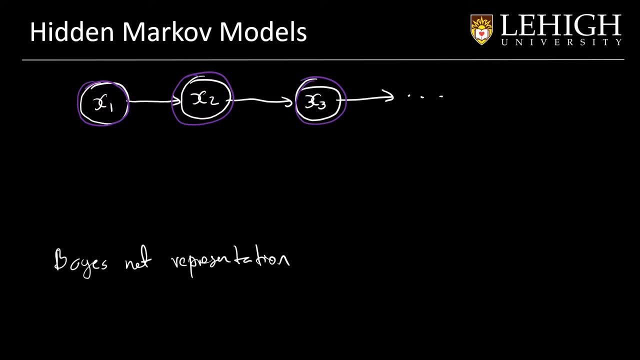 and they will. they, they evolve with time and the. the variables, or in this case the state of the robot is the states at every time step- are independent. that's one of the assumptions of the hidden Markov model and that's the same for the measurements. so we will have some measurements for every time step. we 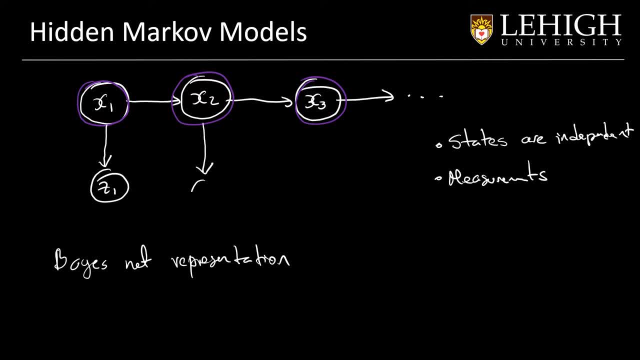 have measurements and actually this is, we have access to this variable. the only problem is like this variable has some error and, additionally, we have also control inputs and the control inputs can only influence the net, the the current time step. they cannot influence, like, the future of the past. okay, so we 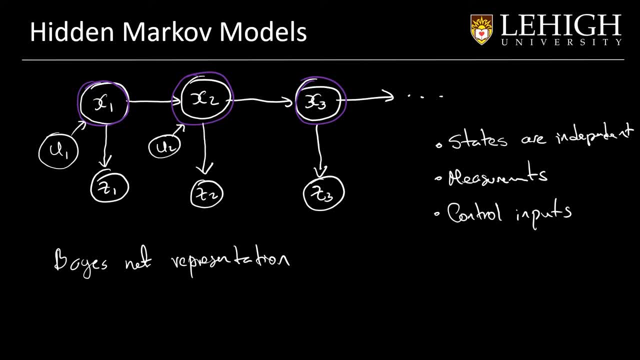 have you want you to, and every for every step, we have a control action and we can also have a measurement of the state. okay, so what we want to obtain, or what we have now to obtain, that is the probability of xt based on the, the state in the previous step and the control input. right? so what if we combine these? 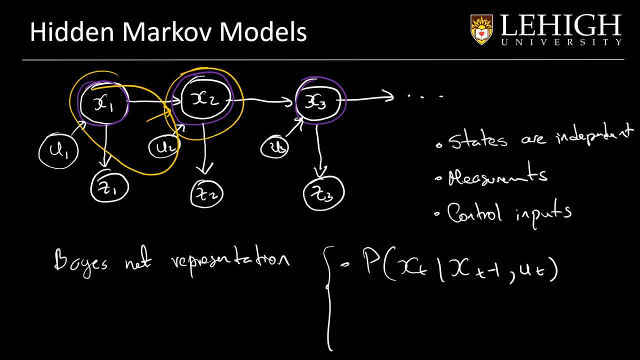 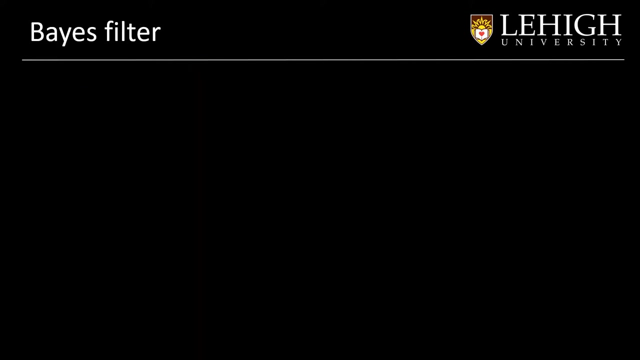 two values to obtain this value over here. that's the first part and the. the second part that we can obtain is the probability of xt, given zt, which is here. basically this part over here. based on the measurements, we can also estimate the, the variable. a specific model of the hidden Markov models is the Kalman filter, which is within the family of the. 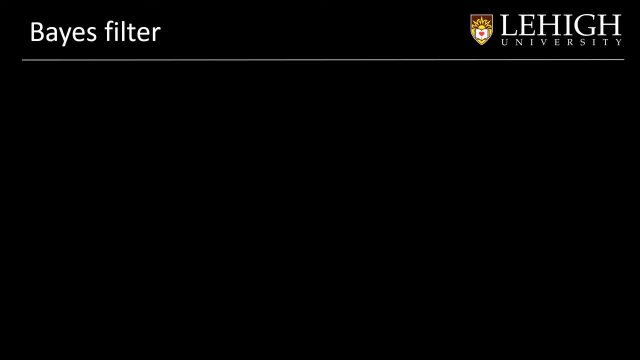 Bayes filters, mainly because they use the, the Bayes theorem, to estimate the, the hidden variable, based on the evidence. the Kalman filter has been very important in robotics and in many sciences. just to give a fact, the spacecraft that went to the moon for the first. 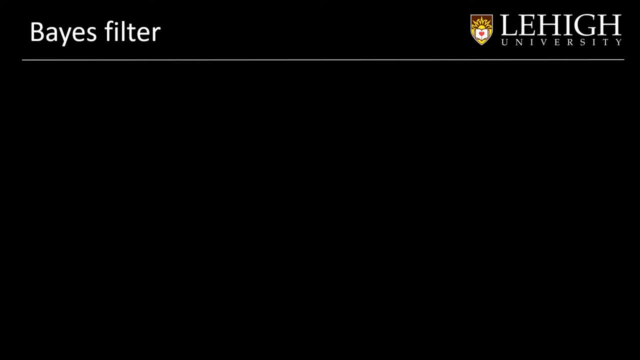 time when the first man put a step on the on the moon was based on the Kalman filter. we will see that there was a slight distortion, but we are able to estimate on it exactly. the equation is very simple and they were able to implement that, implemented in the computational power that 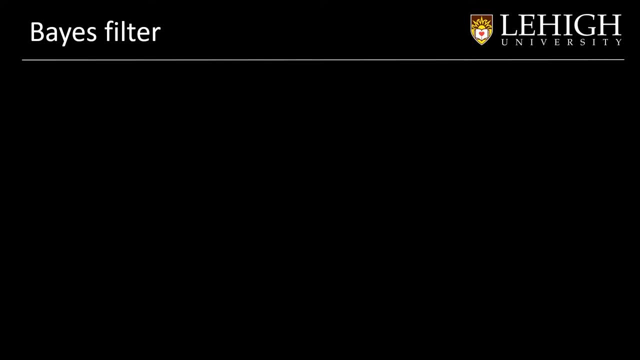 they have in the moment, we, which basically what we have in a simple calculator these days. the assumptions of the Kalman filter are basically that all measurements, estimations, motion, all the beliefs of the state are gaussian distributions. so if we have alreadyücke, so Neil Morey, and registering the function power of that meter in was that was the, simply the various functions. example: works now the joules, or that measurement function is given to the constant cake, blockchain is normal. or the hours and those whoài is thus possible that�н. 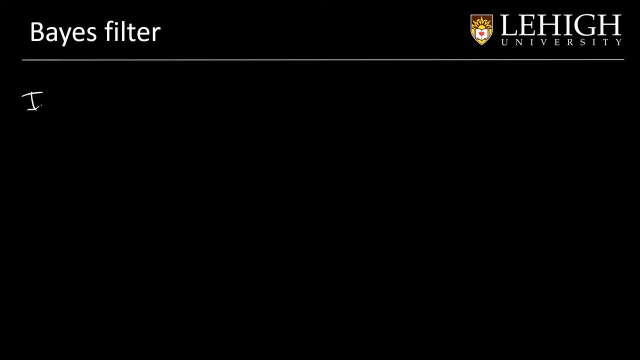 So let's start with the initial belief of Xt, which is a normal distribution with a center in the location that we think where the robot is and covariance that's associated with the error or our estimation of where the robot is. So if we want to see it graphically, this is kind of the coordinate system. 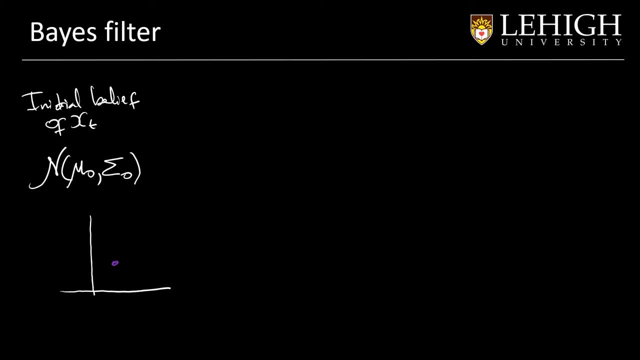 Our robot is here, or that's where we think that the robot is, But we are not sure at all. so maybe the robot is around here, Around the circle, or, if we have a pretty good estimation, we can say that it is around this ellipse, And the ellipse is associated with the covariance matrix. 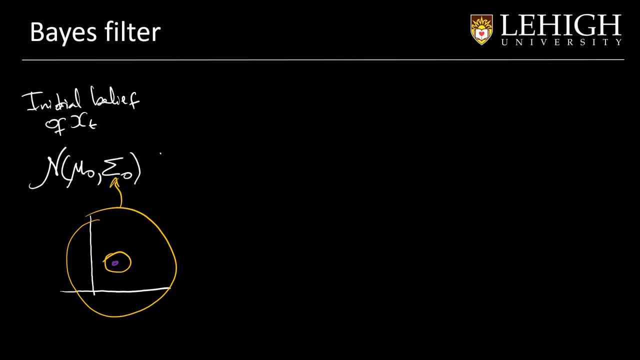 So the first step is the prediction step. It's the prediction based on motion, Like when we walk some steps And we Try to estimate where we are based on the number of steps that we counted. So for that we use the control input and the previous step Right. 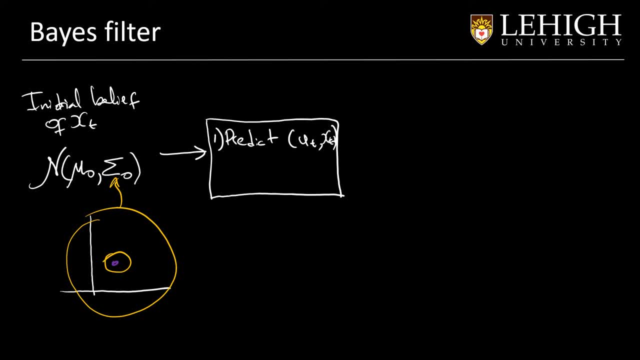 And this prediction is based on a normal distribution that will model the motion And we will have Mu? t. Let me write down This is the mean: that we put a bar just to say that it is based on the prediction And we have a covariance That is also based on the motion model. 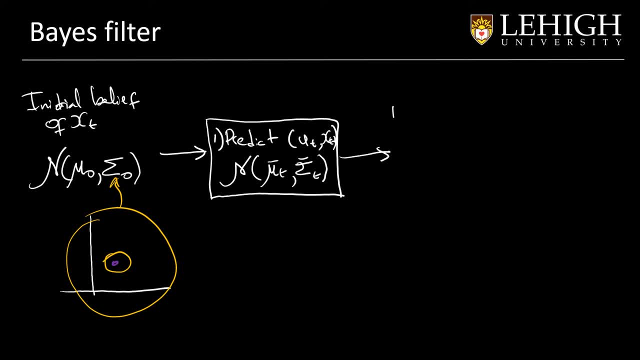 Our next step is the correction. We walk some steps And now we need to correct them. We correct them based on the measurement that we obtain Okay, And the result of this correction, We will be also A normal distribution with estimated mean and covariance Right. This is the output. 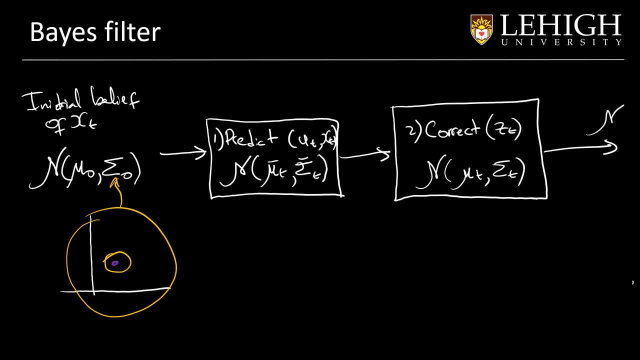 The output will be the normal distribution And if we continue doing this process, We will have a good estimation of the robot. So the first step will be Having the robot with an estimation of where the robot is. We apply a control input And the control input will guide us about where the robot can be. 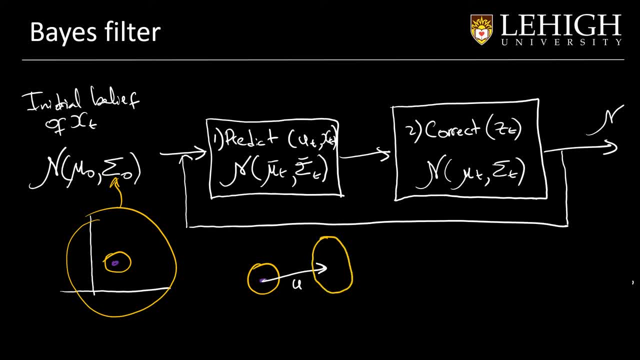 But the error might be. Actually, the error is bigger than in the beginning, At least. the good part of this is that We know that we are around this area, But, for example, we will not be behind. This is wrong. This is not. We will be inside That area. 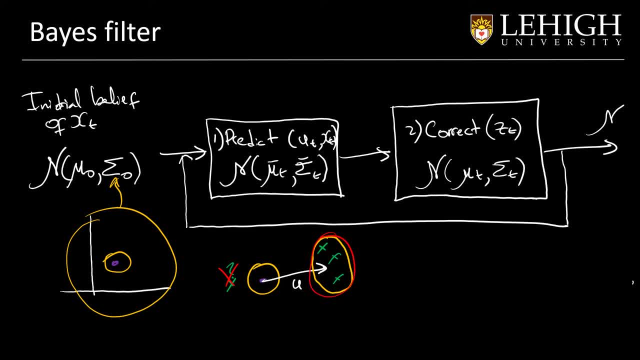 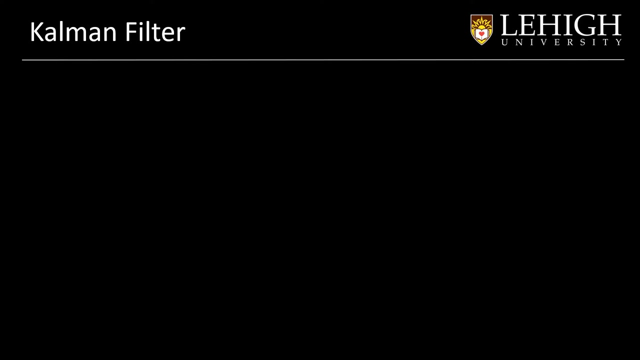 Okay, And in the next step, What we do is to combine our previous estimation Of where the robot is And the estimation of the That comes from the measurement, And we will combine it to improve Our estimation of the robot. So, as I said, the Kalman filter is based on. 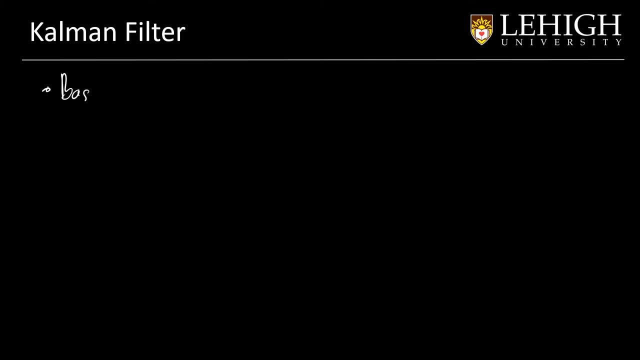 Gaussian distributions, Gaussian distributions- Everything is a Gaussian distribution. We have that t-1, We have that xt, We have zt, And even the model of the motion Will give us a Gaussian distribution. When we operate with the Gaussian distributions, We multiply them, We add them And the result is also a Gaussian distribution. 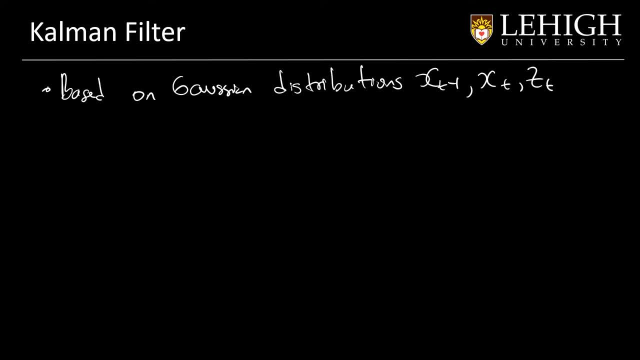 That's a nice property. They are close. So we have another assumption. The other assumption is that Our system is linear, So we will call it a linear stochastic model And I will write down the general equation For what we assume in the Kalman filter, Which is that the new state 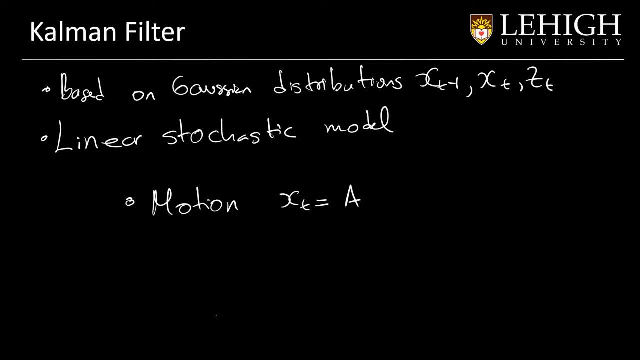 Is equal to a matrix That relates the previous state And the new state, Plus a matrix that relates the control input And the state, And, finally, an error, Which is a normal distribution. This error follows a normal distribution. Okay, And we have a measurement, Which is basically The variable z. 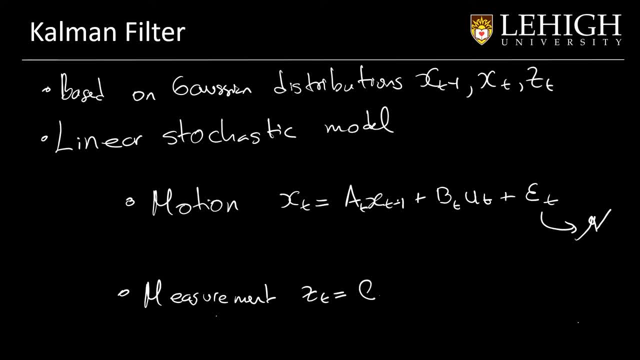 That relates the A matrix, That relates the inputs Or not the inputs, The state And what we can see from the state Plus an error. Okay, This is the general Kalman filter In our case. We will simplify this And we will just assume that The control input is the velocity. 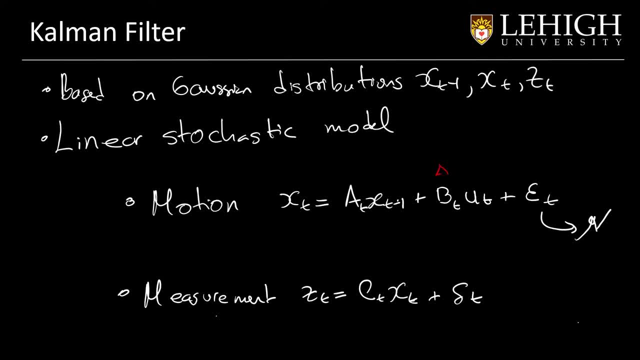 So we just need to multiply this by Delta T And we will obtain the desired state, And A- The same variables of the previous state- Are the variables of the new state. So this is the identity matrix And we will keep this, The error, the way it is For the output. 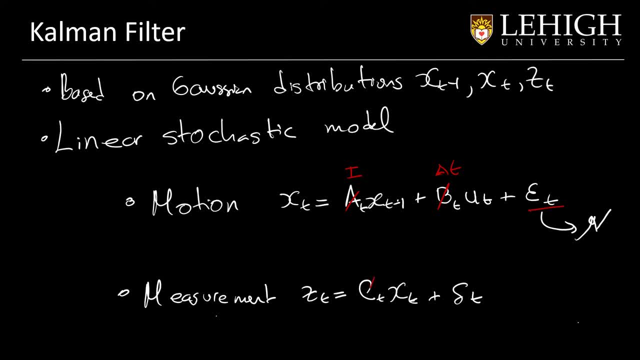 We will assume that We can see all the variables Of the state. So we will have I, So we will have. In this case, We will study like A simplified Kalman filter Specifically for holonomic robots, If we. The important part is like, If we know the state. 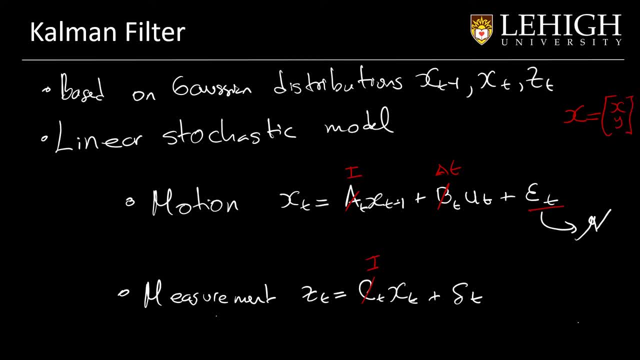 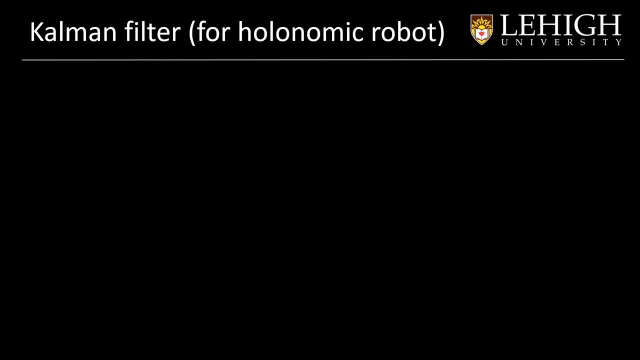 That is X and Y, And we can control its velocity. If we have this type of model, We can apply multiple simplifications In the Kalman filter. So our, As a result, What we will have is that Our motion model. We will represent it by The mean of a Gaussian. 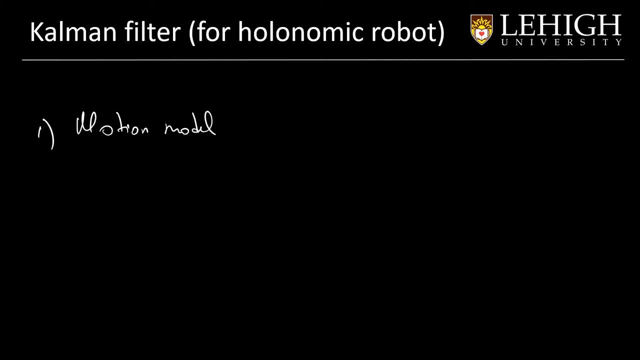 This is a Gaussian With mean Equals to The mean, The mean Plus The control input. Here there is a delta T That we can assume. that is one And we need For the Gaussian distribution Of the normal distribution, We need covariance, So the covariance Will be equals to The covariance that we had. 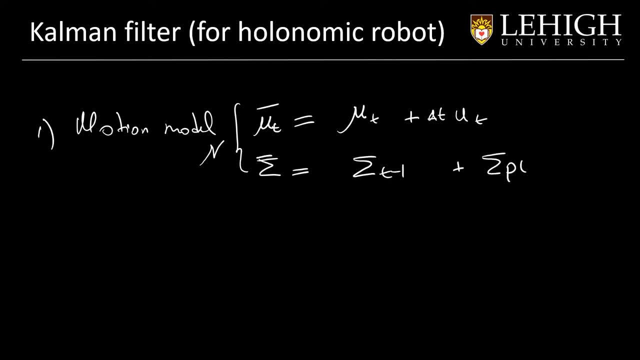 Plus the covariance that we had Because we were moving. So that is the covariance of the prediction. So we will have this And second We will have the measurement model. This is the second step of the Kalman filter, Where we do the correction. The important part here, And this is what they call the 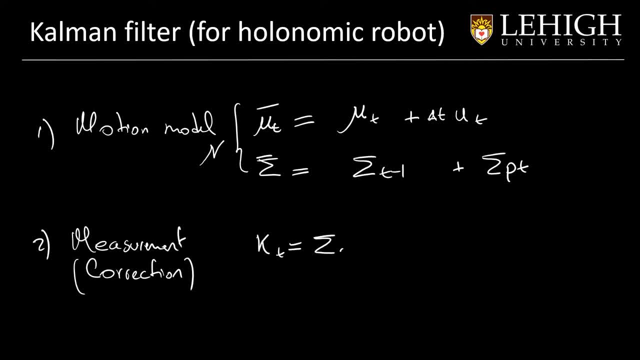 Kalman gain, Which the equation is equals to The covariance that we obtained from the Motion model Times, the inverse Of the Of adding The, The covariance that we Had from the motion model, Plus the covariance of the Measurement. Okay, Every time we read, We try to identify the location. 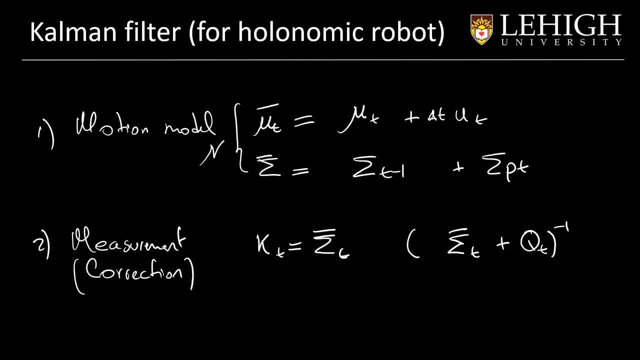 Using a sensor, We will have an error associated And we abstract that with the, With the covariance matrix that is here, And we will use this Kalman gain And to obtain the normal distribution Of the, Of the That represents the, The location of the robot. The good part, since we see, like here: 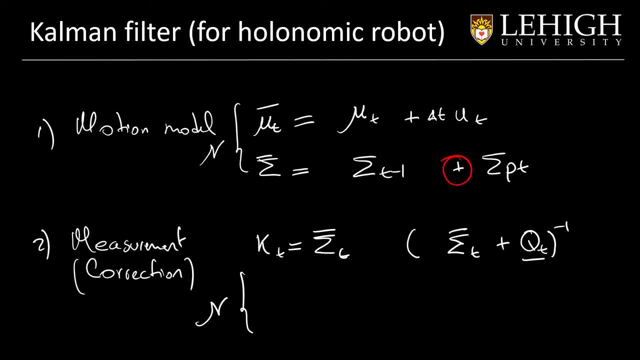 Here we are adding And here we are multiplying. The difference is like When you add two normal distributions, They will start to spread, So the error grows. But when you multiply- And that's what the gain- This is called the Kalman gain- Is, because the error will be. 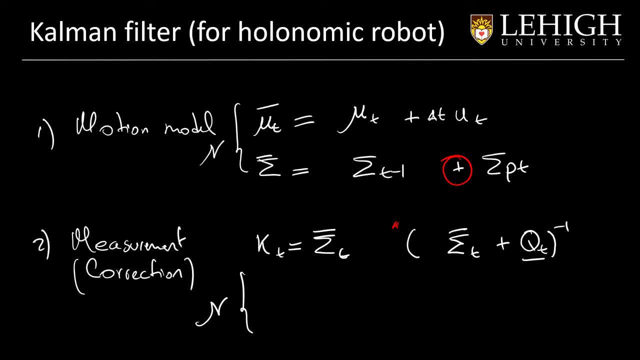 The error will be reduced Or the estimation Will be reduced, because you are combining Two different types of Estimations. Okay, So our result Will be The mean At time. t will be Equals to The, The mean of the previous, Of the previous normal distribution That comes from the motion model. 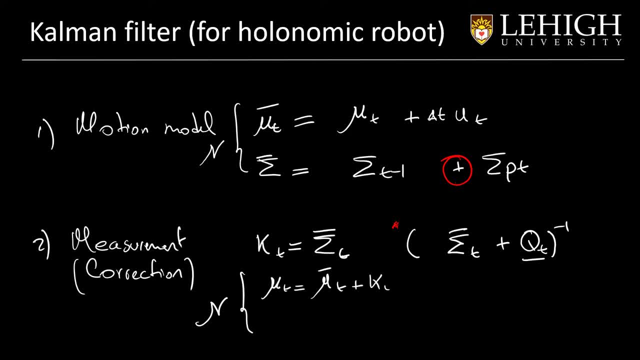 Plus the Kalman filter, The Kalman gain. That That Relates the measurement And the The previous estimation. Okay, Now The covariance will be equals to I minus Kt. This is Kt. We can see that these equations Are in the book And the derivation of these equations. 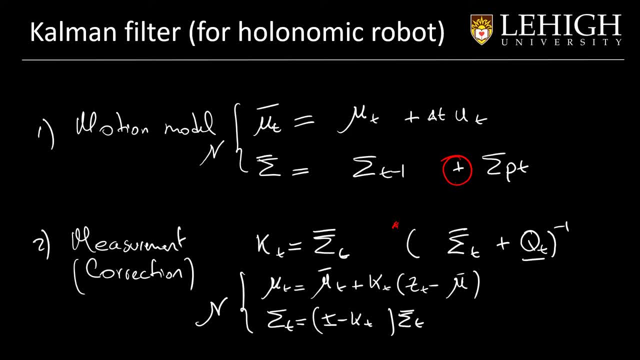 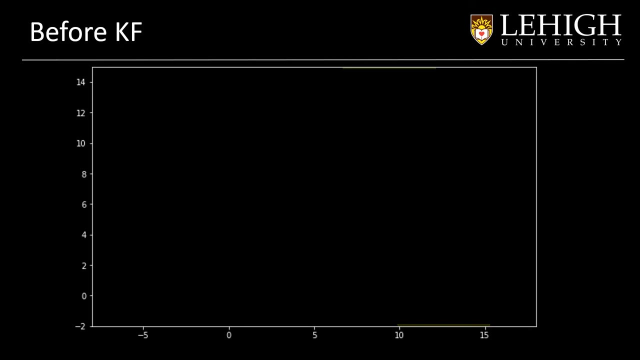 Are pretty interesting. We are going to focus on the Intuition, On how they work, And later we can study the derivations On how to obtain those Equations Based on the estimations, The prediction model And the combination of them. So now Before the Kalman filter. 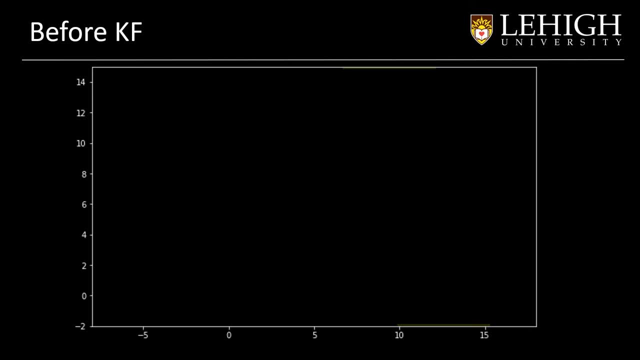 What we had was an error that was Accumulating. So Let's see that we have We start here And we move In this way, Then we move in this way, Then this way, Finally this way. Right, And we had that. the error was Accumulating, Just to give an example. 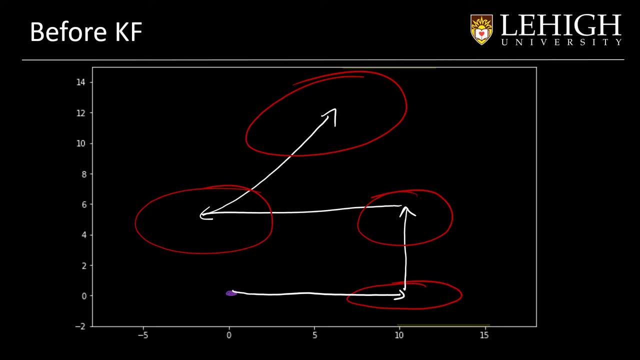 We can have The real robot. The real robot was very close to the, To our estimation, But when we move forward, It moved to here. It moved to here Because it doesn't even follow perfectly, Because there is an error In the control input, And it moved to here. 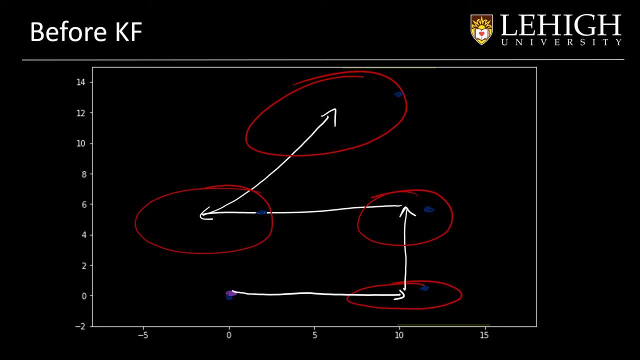 And, finally, The robot will be here. If we see What we can see From the measurements, The output that we get from the measurements Will be something like this: This is- This is after the simulation- We can have this And it says that the error will be Around this. 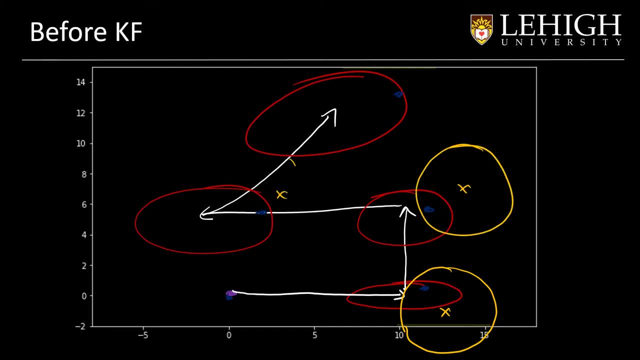 The second measurement will be here, The third measurement Will be here And the fourth measurement Will be this: If we see, If we use the, The, The odometry, The error is pretty big. But the real robot is still inside The range Or the 90% Of the. 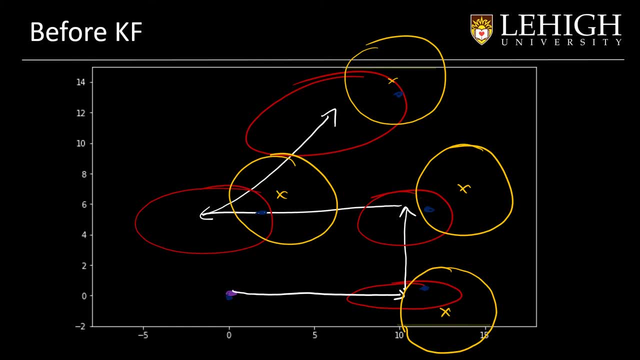 Of the Area that is covered from the Gaussian distribution. Now The problem is with the measurements. Like the measurements Don't change with time, They are kind of constant, But they are still big At every time step. Let's see what happens If we use the Kalman filter. 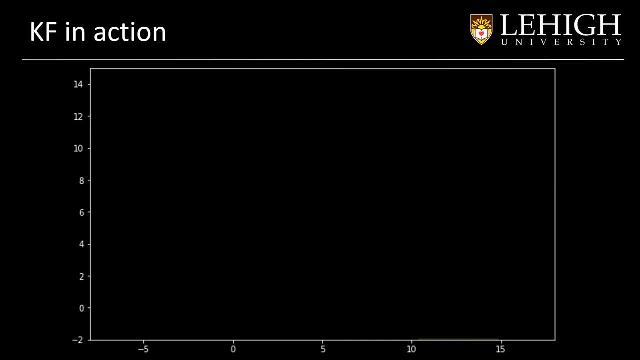 Now let's apply the Kalman filter To combine the information That we have For that. we will start saying that Our robot is in this location. It will apply A control input That goes in this way, And, since there is an error Associated with the motion, It will fall in this point. 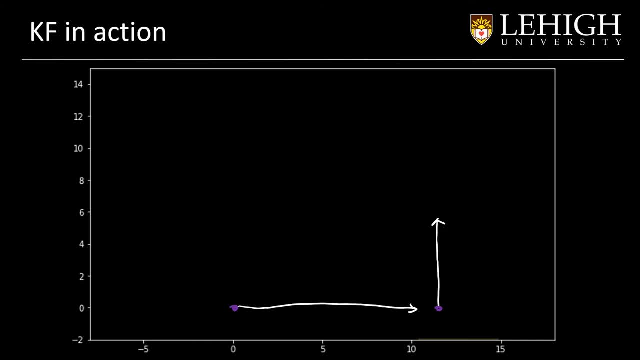 Now it will Apply a control input here And it will fall here, And we will repeat That process, Always taking into account That there is an error in the motion. So This is what happened in reality And The final location of the robot is here. Ok, So From the first. 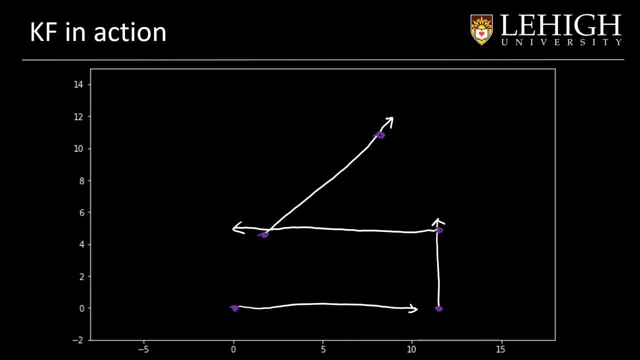 Odometry. From the odometry, What we get is that We will be Around this location, Ok, And Our measurement Will be This here, Ok. So this is pretty bad, And we had A very small error Based on the initial Localization, And now it grows. If we continue, We will have that. 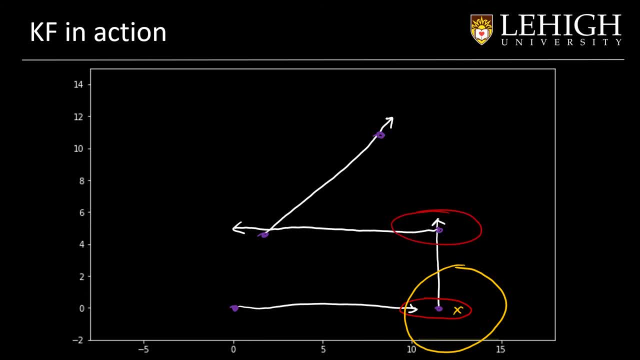 The localization error grows Here And The estimation Will be around here. The error will be: This will be the error, And if we apply The Kalman filter, What we will obtain Is that The estimation, Our estimation, will give A location around this area, And that is based on. 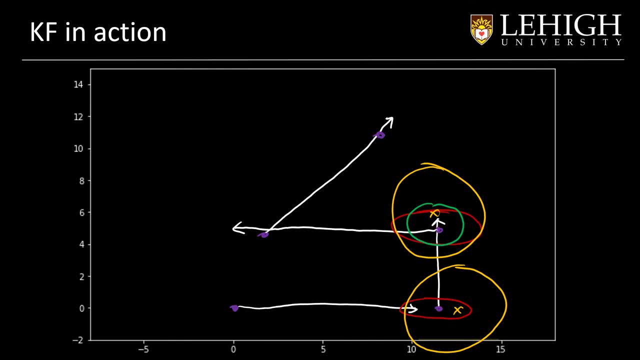 The covariance matrix. Now we see that The error is Way smaller than The bigger. The initial Error of the, Of the GPS. And now We combine the Motion of the odometry With the, With the Measurement of the GPS, To improve our estimation. Ok, It doesn't have to be. 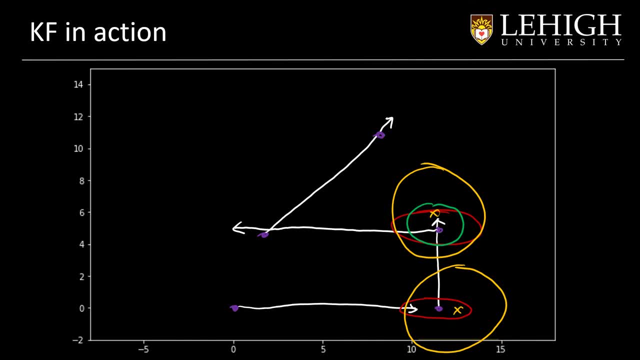 The GPS. It can be like We detect landmarks And it helps us with the estimation. If we continue Using the Kalman filter, We will obtain something like this And finally, Something around here. This is a Pretty small error in comparison To the First initial estimation that we had. 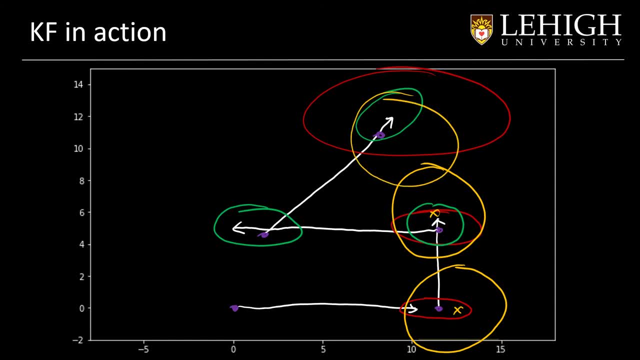 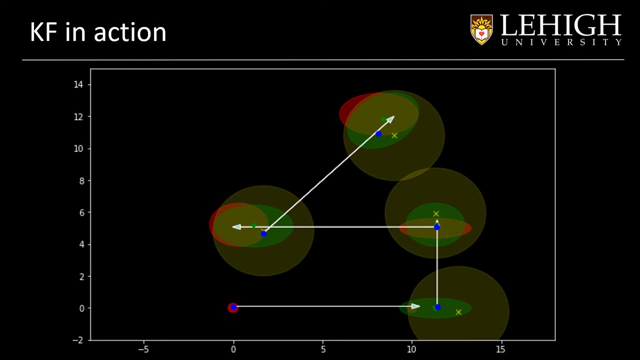 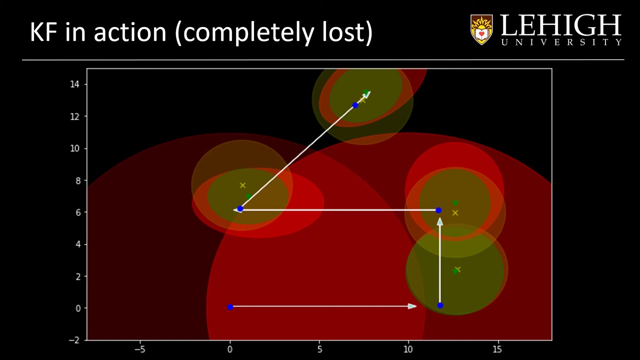 About odometry And the final And the Measurement from the GPS that is always constant. This will be a clean version Of what we will have If we combine them all the time. If we have a case where Our initial estimation is really bad, Like We have no idea about. 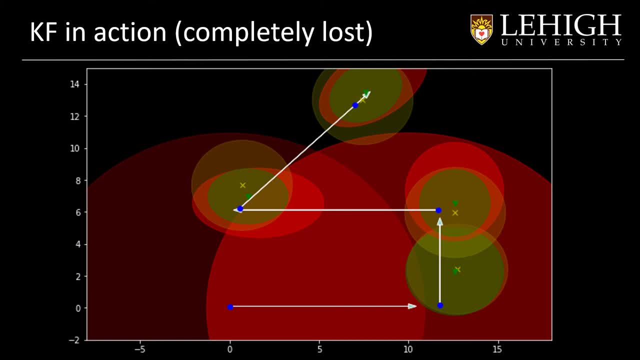 Where we are in the environment. We can make The initial covariance matrix Very big, Such that The error will be Huge. We can place the mean Everywhere And then we will make the Estimation very big. Ok, So we can say that This is the real robot And our initial estimation is there. 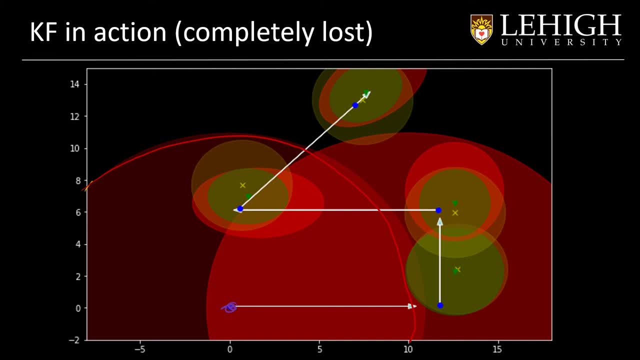 But we have no idea Where it is Based on. If we run the simulation, We will obtain that The estimation will be Getting smaller And smaller Every time we Run the Kalman filter. We will have The information from The odometry And the information from The measurements And, in the end, 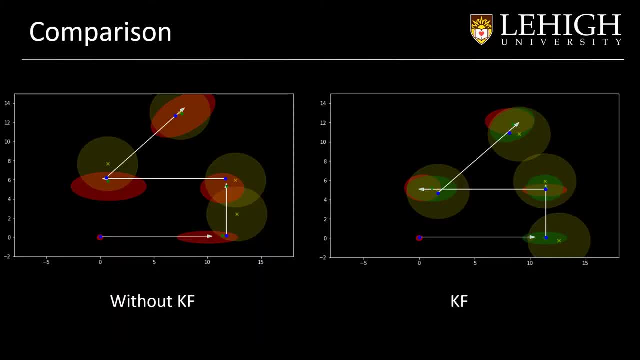 We can see that This estimation is significantly Smaller than The initial that we had. In comparison, We have that Without The Kalman filter The errors are Bigger than If we only use The measurements. They are still big, But if we combine them We will obtain A smaller estimation. 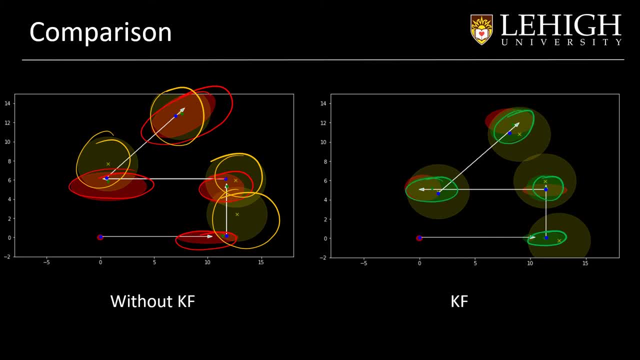 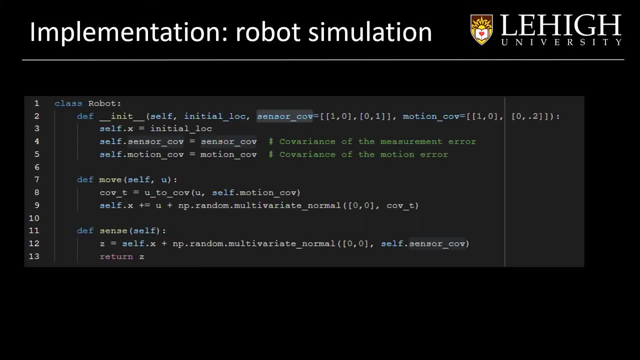 That grows, That keeps being Smaller all the time. For the implementation, We can start creating a Robot simulation And this robot is pretty simple. We just give An initial location When we create it And that will be The state of the robot. We know that The sensor has some errors. 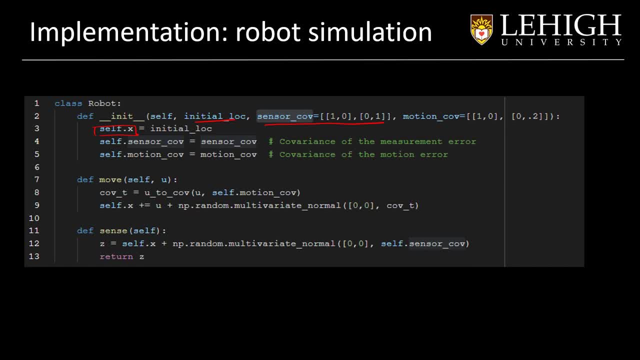 So the covariance Of the sensor Will be given In the initialization The same as the motion. So when the robot Moves It will compute the covariance Depending on The initial motion covariance. Like If the robot moves here It will move like this, But if it moves longer That covariance should grow. 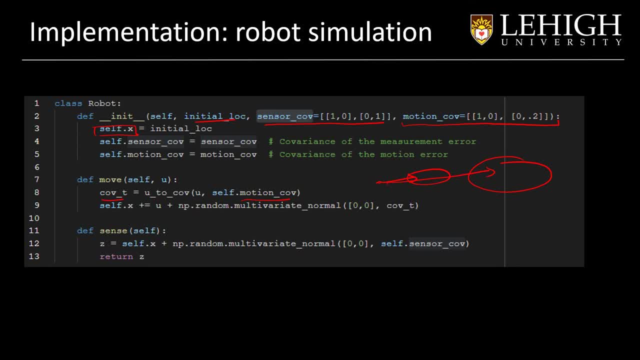 So it will be proportional To the distance And also Proportional to The error In X and Y And the direction Of the control input And the output Will be The. The output will be X. Xt will be equals to Xt minus one Plus Delta tu. We assume that this is one. 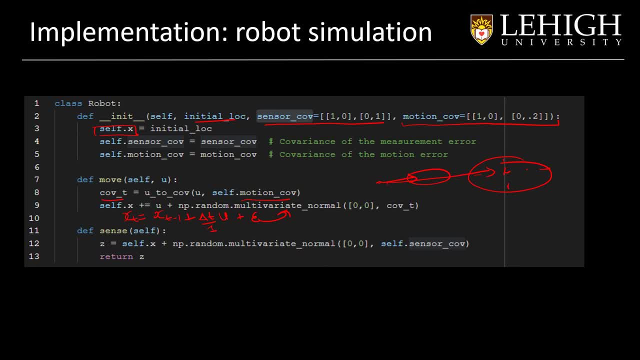 Plus the error, And the error is given by this. So every time the robot Moves it will Have an error. And for the sensing We have a sensor That just gives The value of the Of The actual state of the robot Plus The error. This is the error that we used to call. 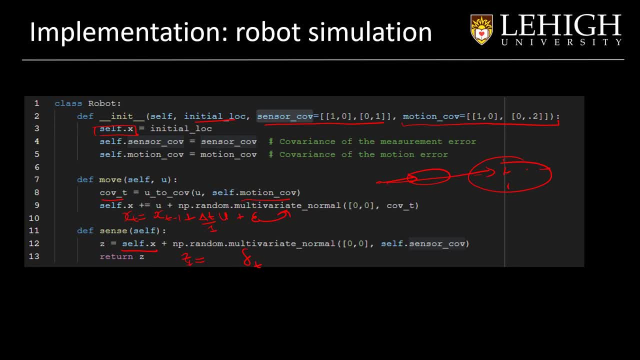 Delta t, So it will be Z equals to Ct equals to Xt, Plus the error, And this is the right way That we obtain A Gaussian error. This is a pretty simple Probabilistic robot That moves With an error And it also gives The location With an error. 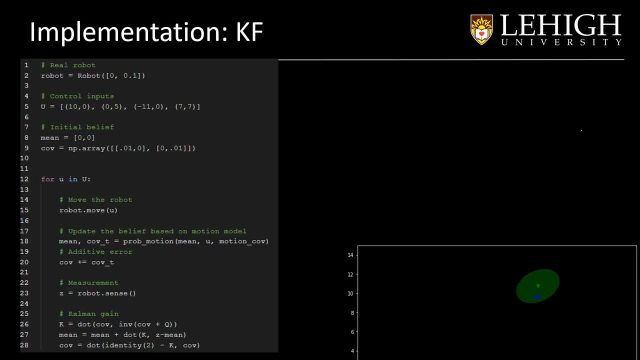 So now The implementation of the Kalman filter is pretty Simple. actually, What we have is that We create our simulated robot. We don't know how that robot moves Or what it gives us, But we have The model of its error. That's something that we Have to be aware. 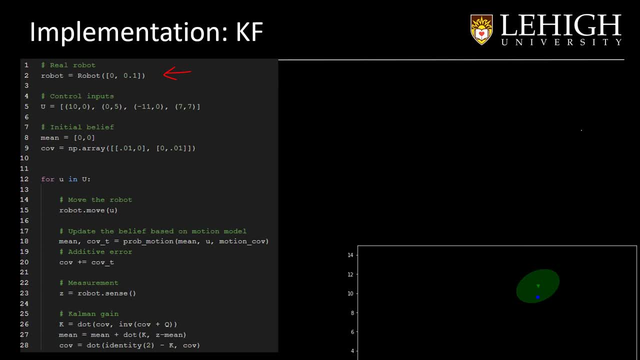 Here is: Our predictions will depend on How good, How good our models Are, how close they are to the Reality. Okay, so We will use the same constants, And Here, when we have the control inputs, Is where we are going to start Moving around. And now, This is our initial belief. 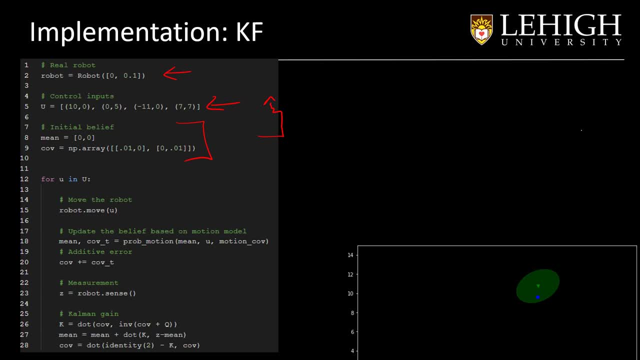 Of the robot that is very Accurate, And then the robot will start To move. For every time step, for every control action, Our robot will move And now, Based on that motion, We will have our Prediction That uses The time Of the previous step And the control input. 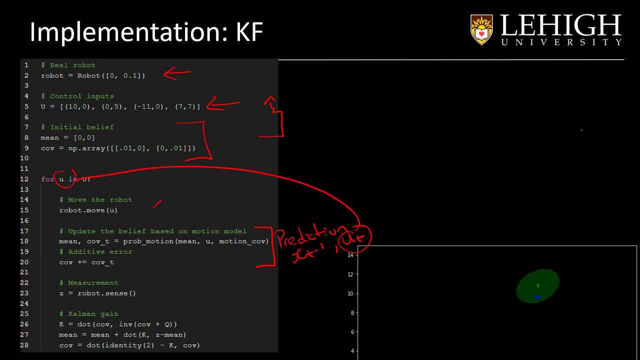 This is the control input That we obtain over here And We said that The error will accumulate. It will add from each Control input to the next one. Now we obtain The measurement And we apply The Kalman gain And we obtain The estimation Based on the measurement And the Kalman filter. 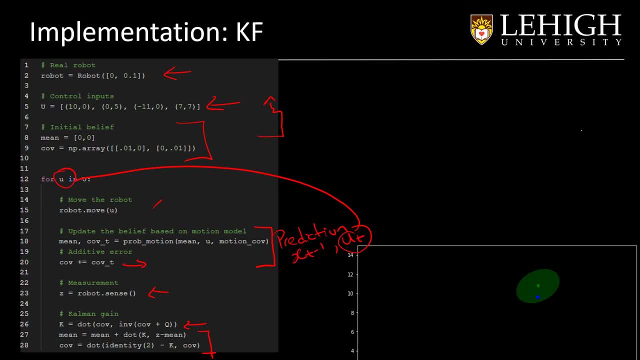 Using this Method multiple times, We will obtain That our Current Estimation is very close To the real one. This is just an example. After running this code, We will obtain something like this: This is the actual robot And This is our estimation, And this was done after Four time steps. 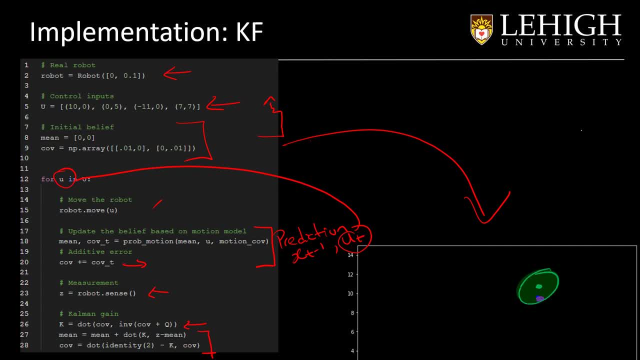 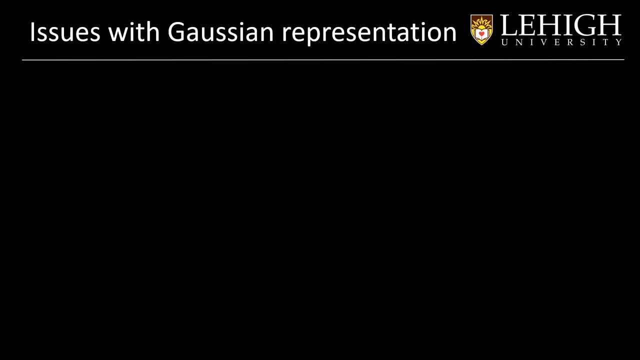 We got a very Close estimation Of the real state. Unfortunately, Not everything Is happening With the Kalman filter. We know that There are some assumptions That really Constrain the real world applications. On one side, The Kalman filter Is very fast. As I said, They were able to. 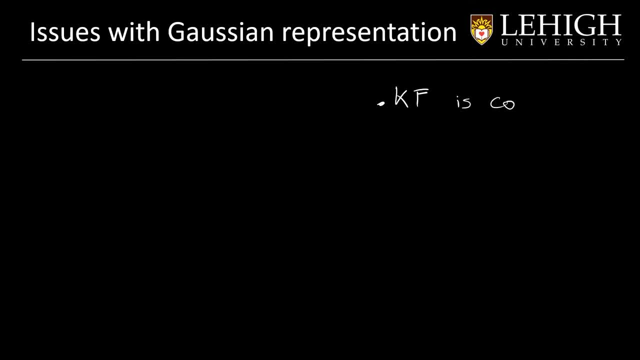 Use it in the spacecraft To go to the moon. So It is computationally fast. But now Let me give you an example. If our robot is here And it moves here, We will expect To be around here. But If there is an obstacle, The probability Distribution that we have, 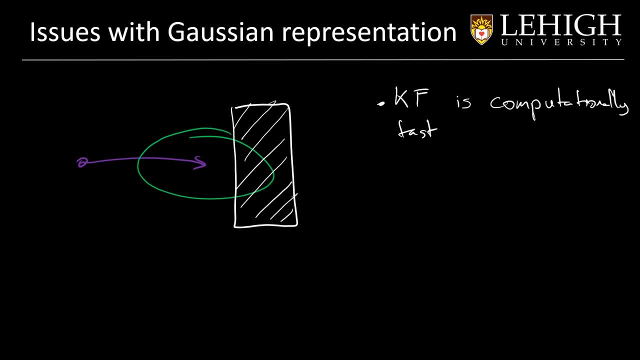 There might not Be like a normal distribution, Because we have to Cut this part over here. We have to cut here, So We will start to study Different types of distributions, Multi-modal distributions, And they don't fit with the Kalman filter. Additionally, The linearity Is another problem. 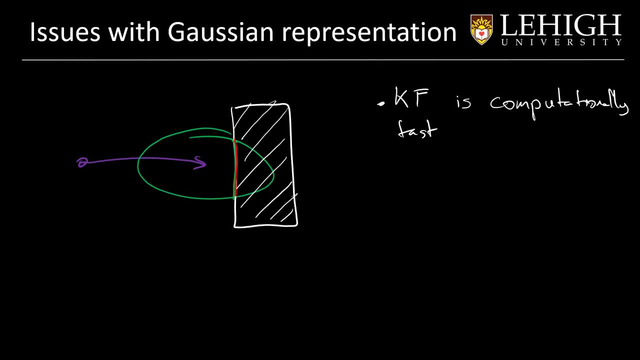 But for that there are some solutions. That will be the extended Kalman filter. So on one side We have that The Gaussian functions Don't adapt To many Real scenarios And we also have An assumption in linearity Does not apply for All types of robots. Okay, So for the 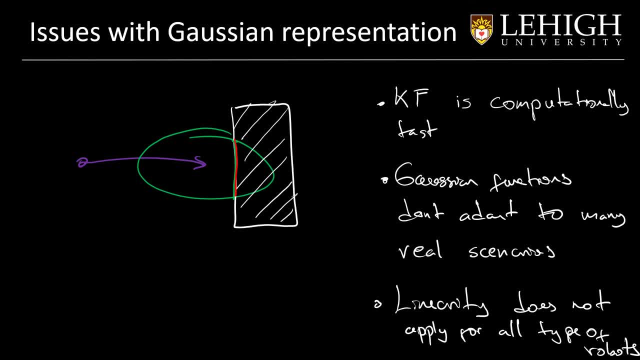 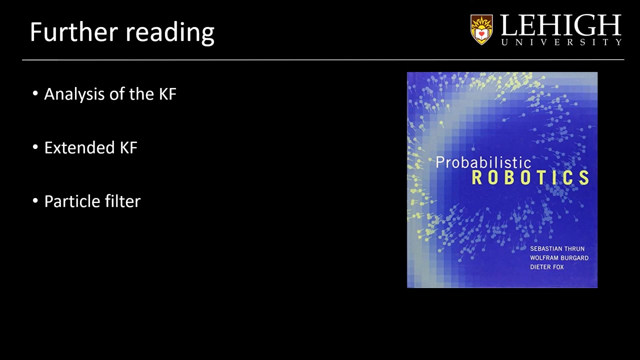 For the last bullet We have something very good That is called the Extended Kalman filter, Which will remove The linearity assumptions And it can also Predict the State of the robot, Based on the Assumption that everything is Gaussian. So for further reading, I really recommend The book Probabilistic Robotics. 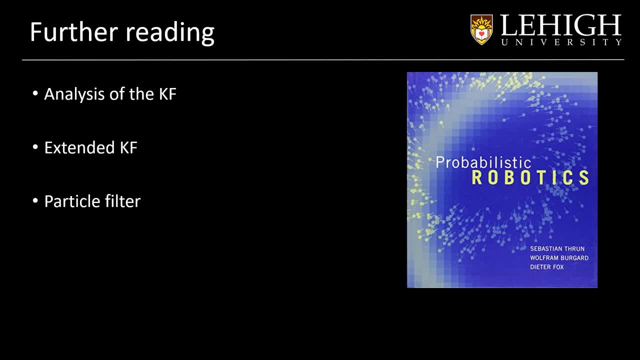 From Sebastian Tron And This is a great book. Like almost every roboticist, Have this book And in this book you can find The whole analysis of the Kalman filter. We can have other methods, Like the extended Kalman filter. We can have probabilistic mapping And this book.